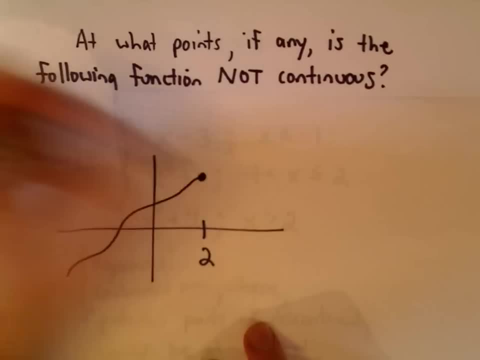 The idea is, you know, maybe that one function is continuous and the other one takes over. so what could happen is maybe it fills in at the right place and just keeps going, Or maybe it starts in a totally different place. So if it starts in a different place, well, it wouldn't be continuous. 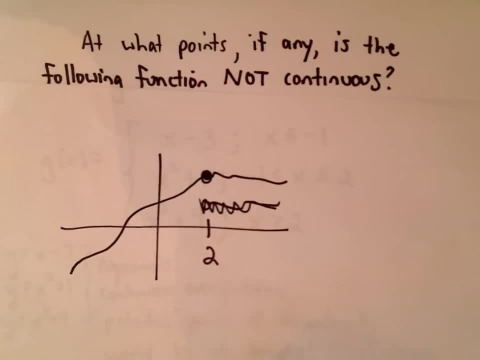 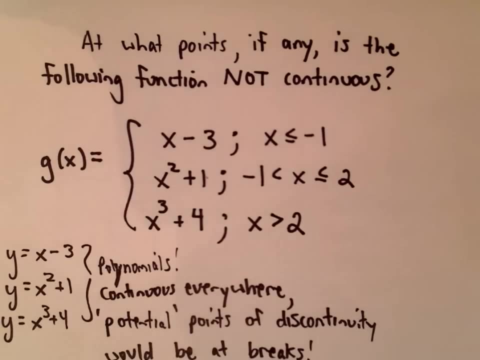 If that didn't happen, you know, and it just happened to take over right at the same place, then it would be continuous. So we're just trying to figure out if they stop and start in the same place, intuitively. That's all we're trying to do. 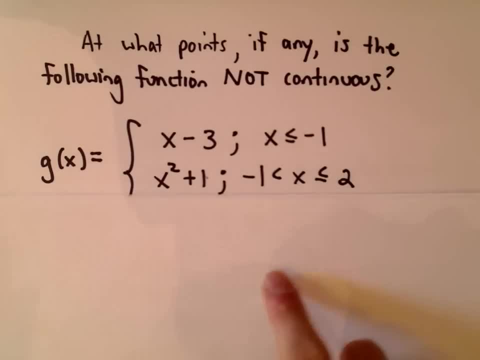 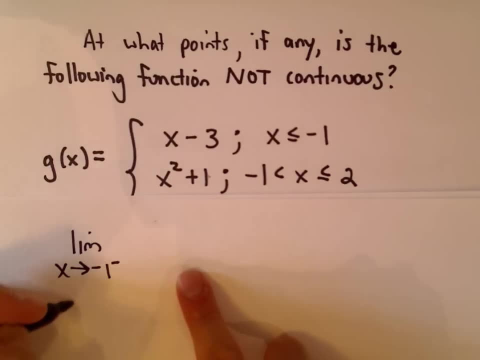 Alrighty, well, to do that, I'm just going to use my limit definition. So there's a break at negative 1, so I'm going to have to look at the limit as x approaches negative 1 from the left. we'll have to look at the limit as x approaches negative 1 from the right. 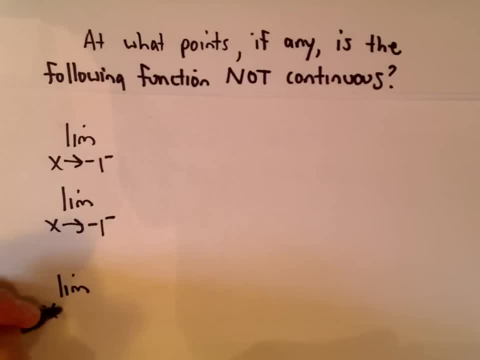 and again. the question I'm trying to answer is: does the limit as x approaches negative 1 of the function? does that equal f of negative 1?? Again, just to go back to that definition at the very, very beginning of the video. okay, 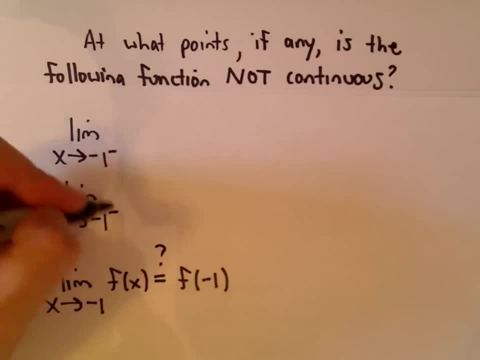 So are those equal? Well, to figure out if they are equal. I don't know if I said left and right both times I put two minuses, so we've got to look at the limit as it approaches from the left and from the right. 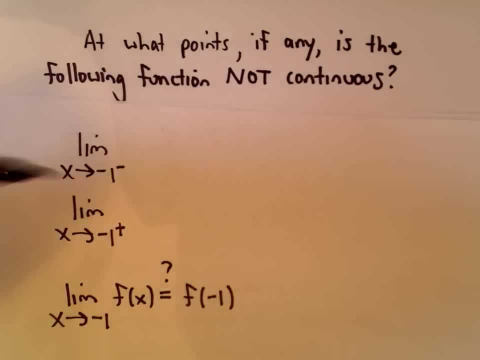 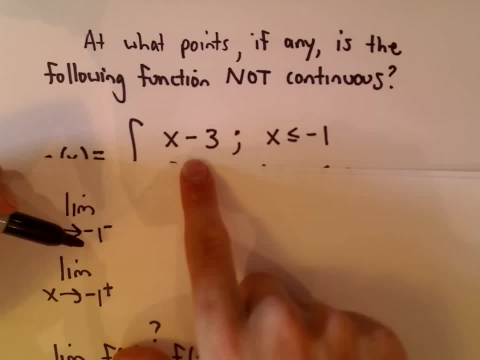 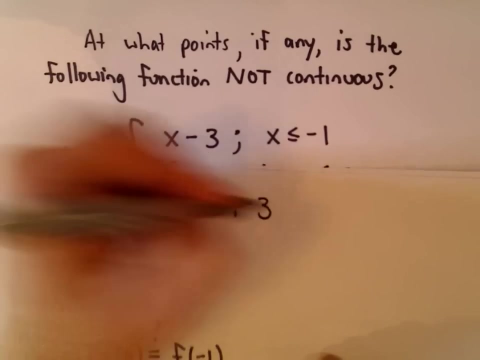 Okay, And we're just trying to answer this question. Okay, so, negative 1 from the left. well, that means we're using x coordinates smaller than negative 1, and that means I would have to use the first formula. Okay, so we would get x minus 3, again, we can just plug this in. we would get negative 1 minus 3,. 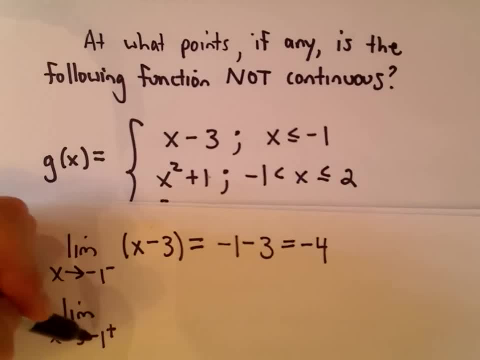 that's going to equal negative 4.. Okay, and then we're going to have to look at negative 1 from the right, so value's just a little bit bigger than negative 1, teeny tiny bit bigger. so then we should use the function in the middle. 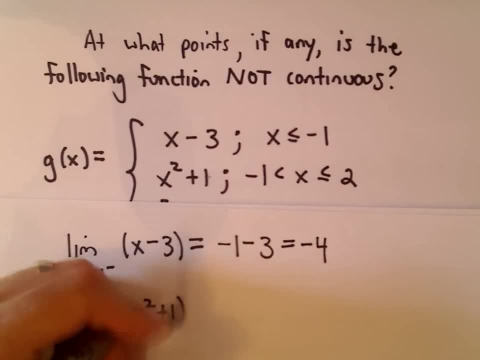 okay, so we'll use x squared plus 1, and again, if you take negative 1 and square it and add positive 1,, well we'll get 1 plus 1, which is 2, and already in this case these can't be equal. 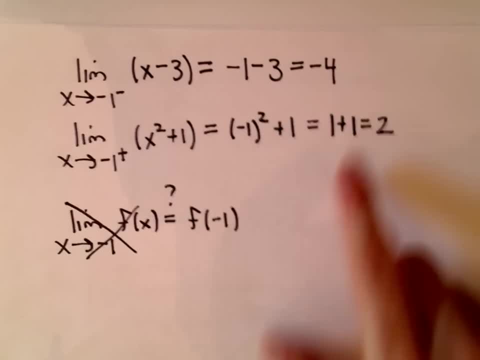 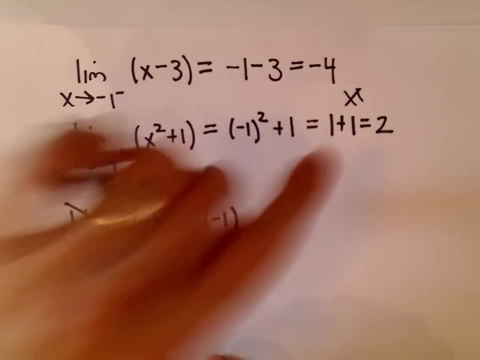 because the limit on the left now okay. so since the left-hand limit didn't equal the right-hand limit, since those aren't equal, the limit simply does not even exist. So if the limit doesn't exist, boom, you're done. 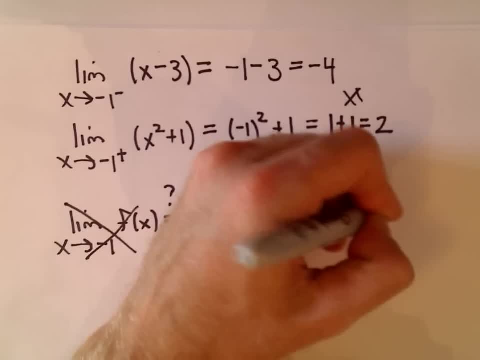 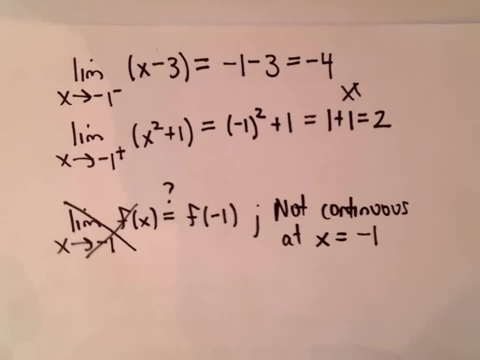 you're done with that one. so now I know it's not continuous at x equals what were we checking? negative 1,. okay, and then we'll do the same thing to figure out if it's continuous at the other break, which was at 2.. 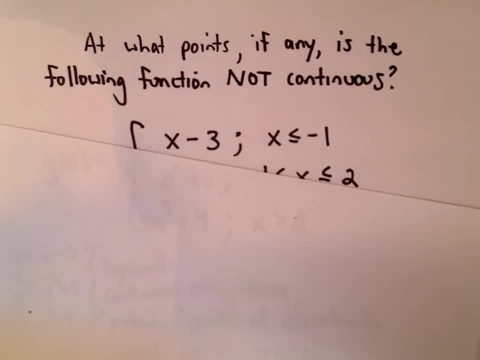 Again, you could graph these, but I think typically people are going to want you know a teacher, a professor in a class. they want to see you use definitions. and again, you know, a graph is an easy way to do it. partly it's just making sure that you understand. 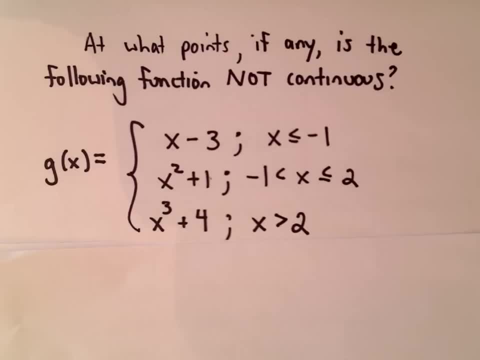 how to compute limits. and again, it's a vital skill to be able to read and understand definitions and make sense out of them. so okay, so now we're going to have to do the same thing. we're going to have to think: does the limit as x approaches 2 of the function? 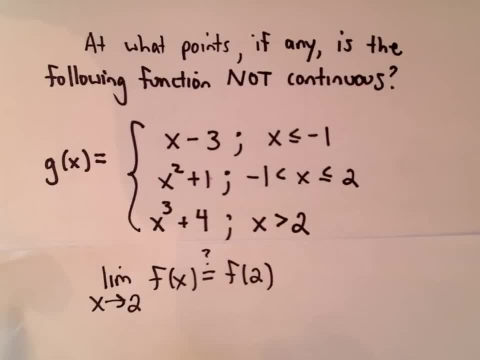 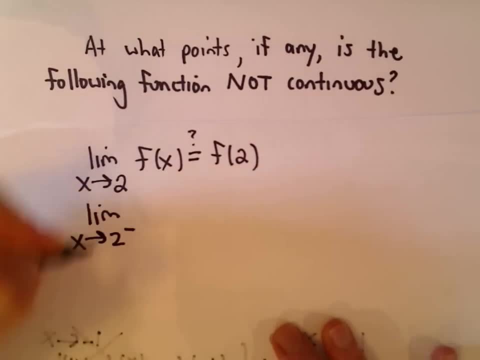 does that equal f of 2?? Alright, well, we're going to have to do the same thing. we'll have to look at the limit as x approaches 2 from the left, and we'll have to look at the limit as x approaches 2 from the right. 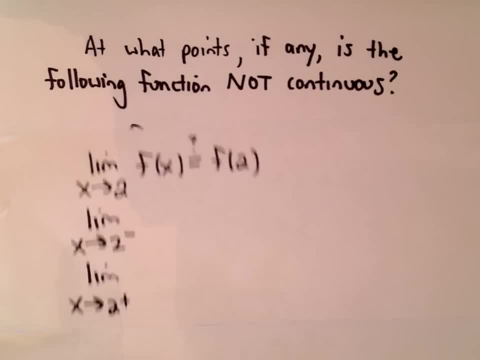 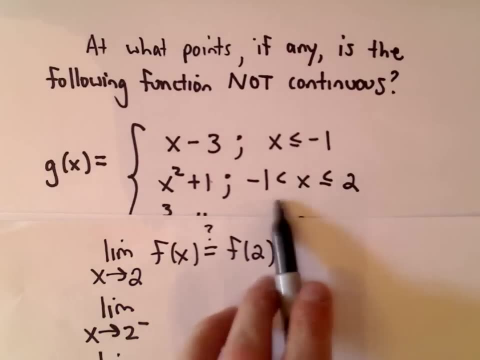 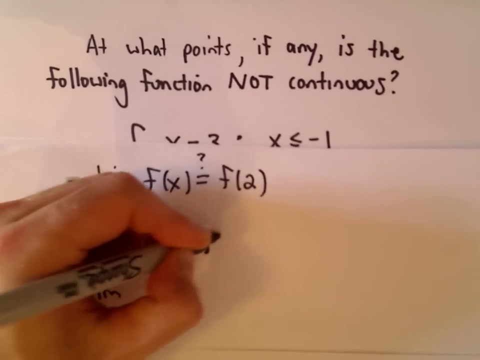 cover up the rest of that there. so 2 from the left, we're taking values just a little bit smaller than 2,. well, again, the second interval is what includes x coordinates a little bit smaller than 2, so we'll plug it into the x squared plus 1 formula. well, we would get 2 squared plus 1,. 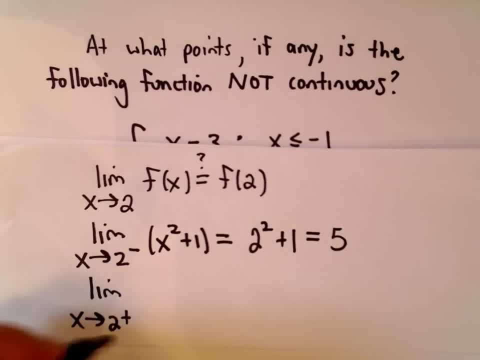 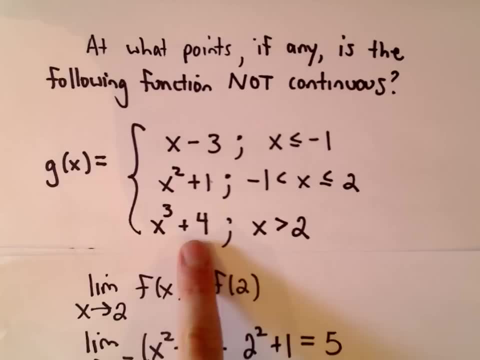 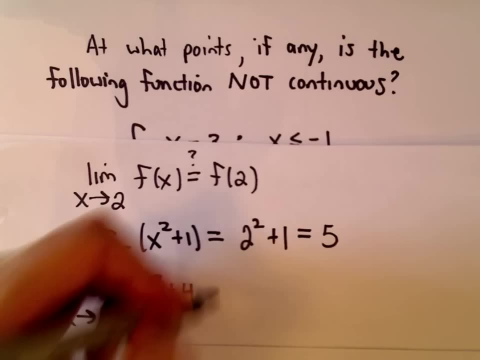 which is 4 plus 1, or just 5,. okay, if we do 2 from the right, we're taking x coordinates a little bit larger than 2, okay, so now I'm going to use my second formula, so x cubed plus 4, and now okay, well, if I plug in 2,. 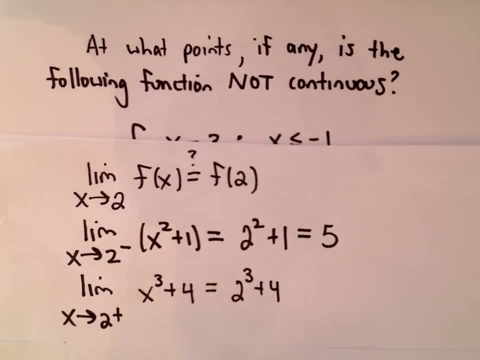 I'm going to get 2 cubed plus 4,. 2 to the third, power is just 8, well, 8 plus 4 is 12, and again, the left-hand limit doesn't equal the right-hand limit. so since the limit doesn't even exist,